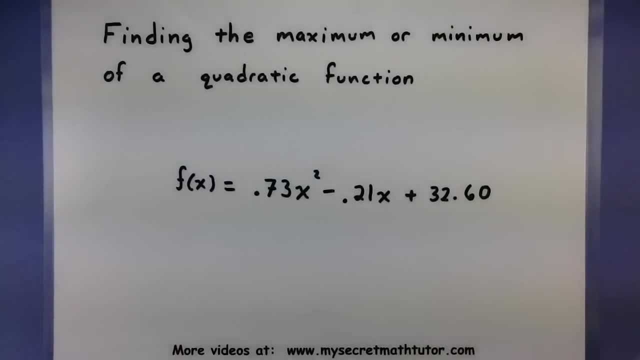 at some of these quadratic functions. sometimes they can get quite complicated. They might have decimals, fractions or a few other things, But finding the min or max is actually a straightforward, simple process if you know what to look for. So let's look at the process and see how this 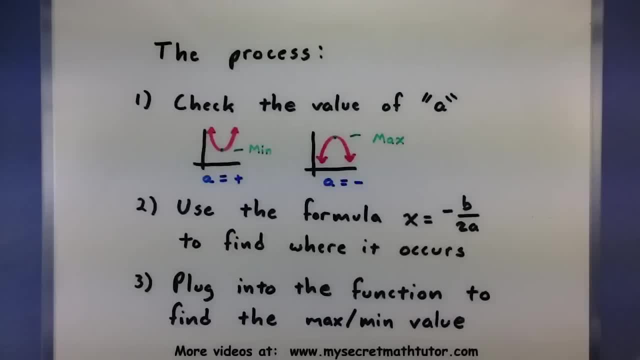 is done? To figure out the maximum or minimum of a quadratic, the very first thing we need to do is check its a value. This is the coefficient in front of the x squared term. Now, what this will essentially tell us is that the quadratic is either facing up or down. Here's how it. 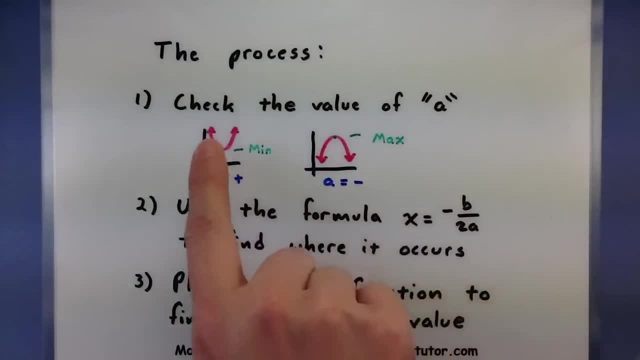 works. If the coefficient in front of x squared is positive, then our quadratic is facing up. That means that it takes on a low value and that it will have a minimum. If, however, that a value is negative, then our quadratic is facing down, and then it has. 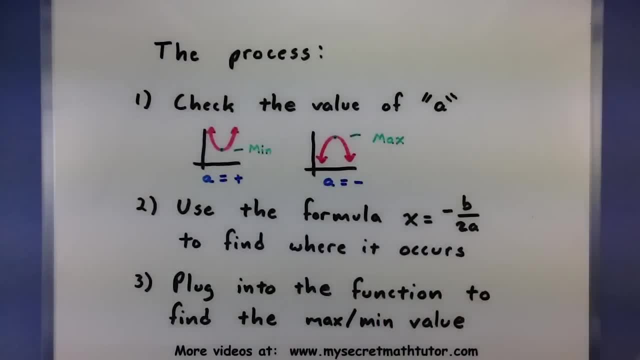 a maximum value. So, in either case, we're essentially just looking for the vertex. Now it's going to really help us out, because for the second step of this, as soon as we know which direction it's facing, we simply use the formula for the vertex to figure out where that max or 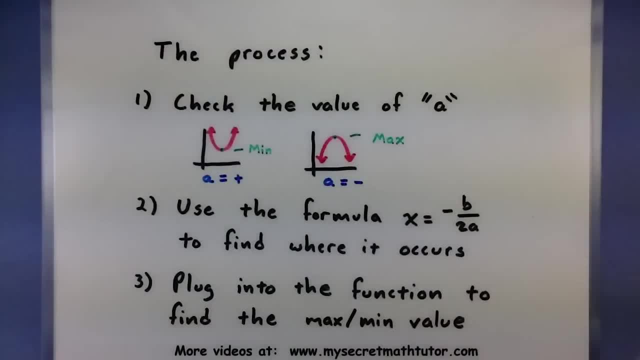 min is located. So we use: x is equal to negative, b over 2a. Once we have that value, we plug it into the function and it will tell us what the value of the max or min actually is. So now let's do two examples using this process and. 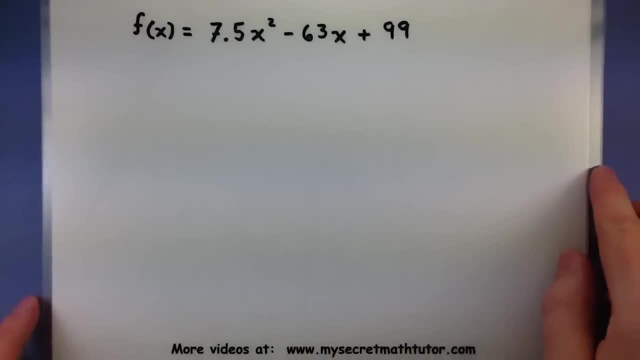 you'll see exactly how easy this is. Alright, so this is my quadratic function, and I want to find the maximum or the minimum, depending on which one it has. The very first thing I do is go ahead and check the a value, So that again is the coefficient right in front. 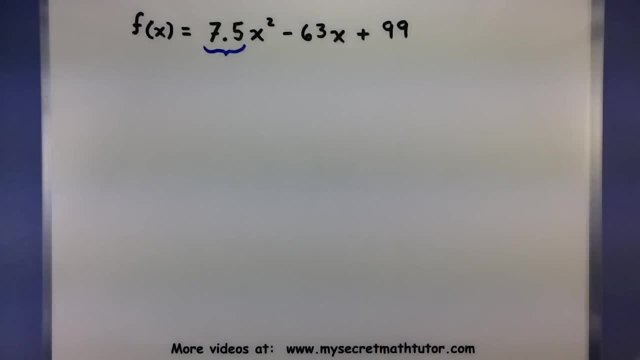 of x squared. As you can see, this thing is positive, 7.5, a nice positive number, And the information I'm getting from that is that my parabola is facing up, So I know that it will have some sort of minimum. 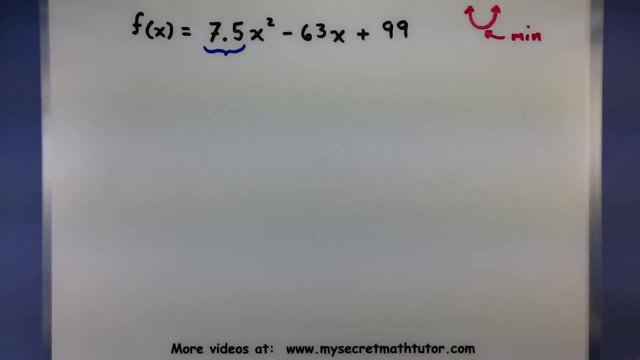 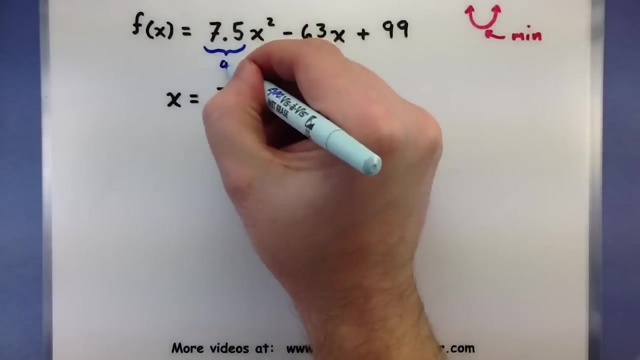 value. Now I just have to find it. Alright. this is where that formula comes into play. So I know the minimum will occur at: x equals negative b all over 2a. So I'm going to use my 7.5 for the a value and I'll use this one in front of the x for the b value. 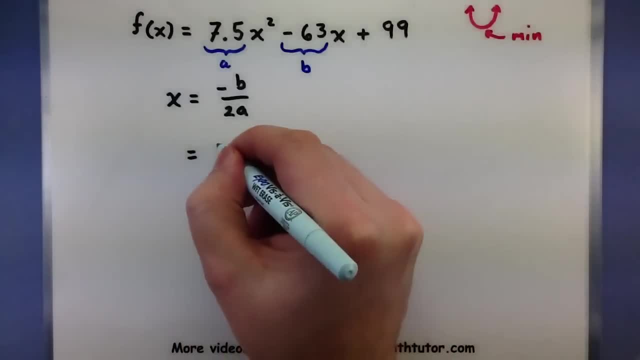 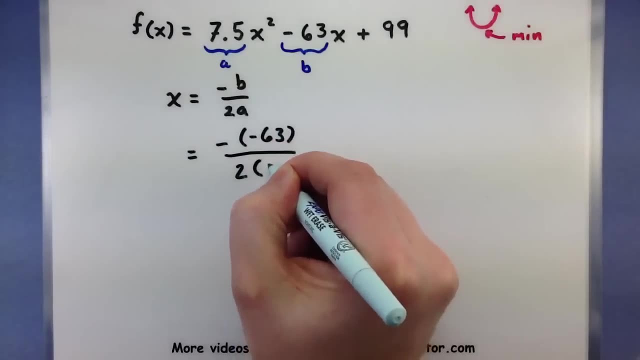 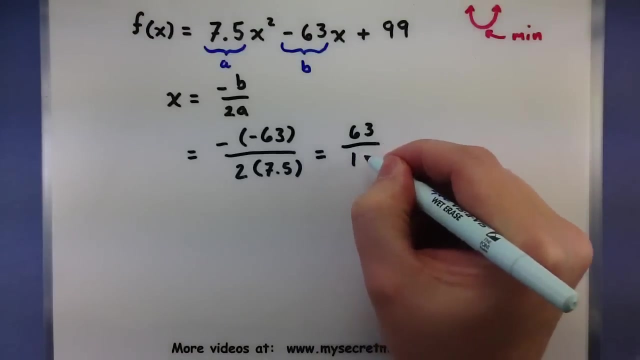 Alright, so x equals negative and we'll use our b value: a negative 63 all over 2 times the 7.5.. Alright, now, this will require a little bit of simplification, but not too bad. So negative times negative will be a positive 63.. 2 times 7.5,, 15.. And it looks like this: 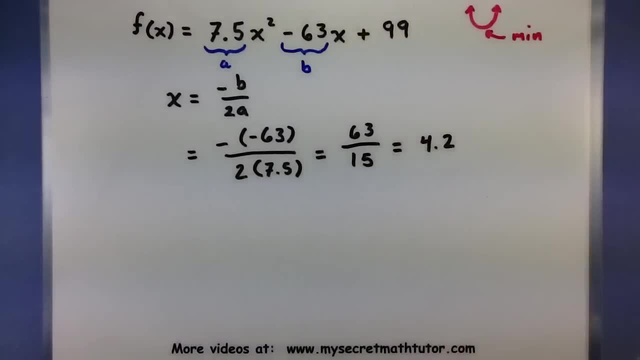 just turns into a 4.2.. Now be careful that 4.2 is not the minimum. this is where the minimum occurs. If we actually want to figure out what that minimum value is, we need to take this 4.2. 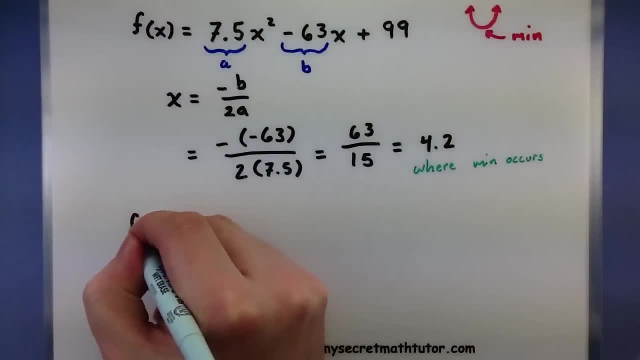 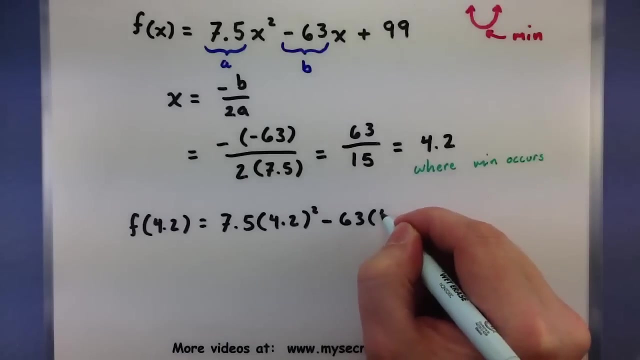 and put it into the function. So let's take our function: plug in 4.2.. So everywhere you see an x, go ahead and put in 4.2.. Now, even though there are a lot of terms in the function, you can always use the calculator. 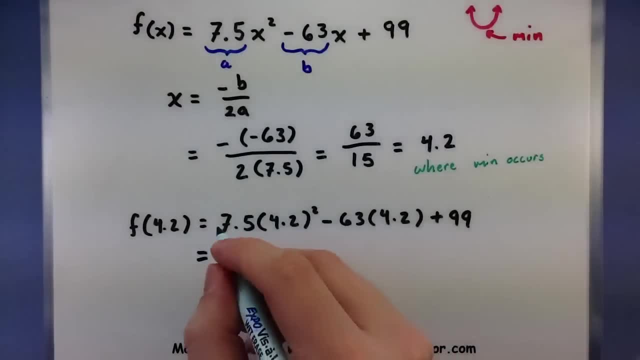 to help you out with some of these calculations. When I did this, I got a negative 33.3.. So now I can say that the minimum value is a negative 33.3.. In case I ever want to know where it is. remember we already found this earlier. it happens. 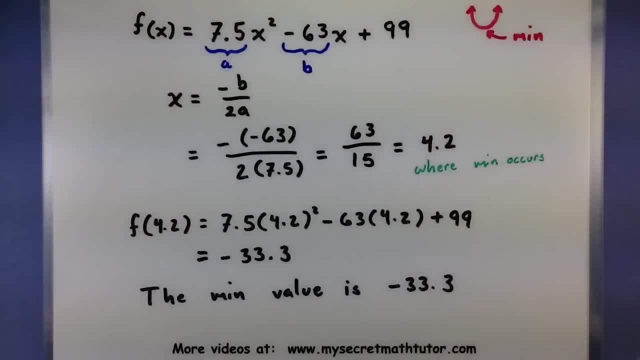 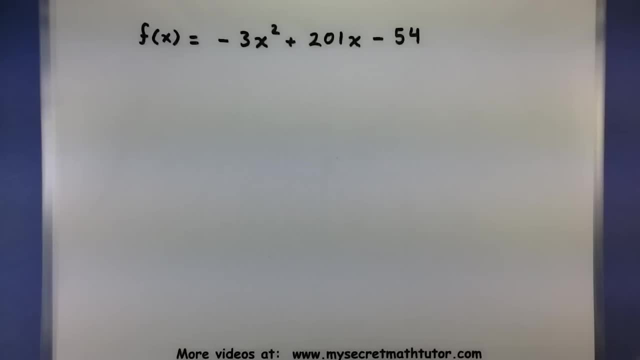 when x equals 4.2.. So the process is pretty straightforward. but let's see this one more time, just so you have it down. Now we'll try it with a negative 3x squared plus 290.. We're getting 1x minus 54.. 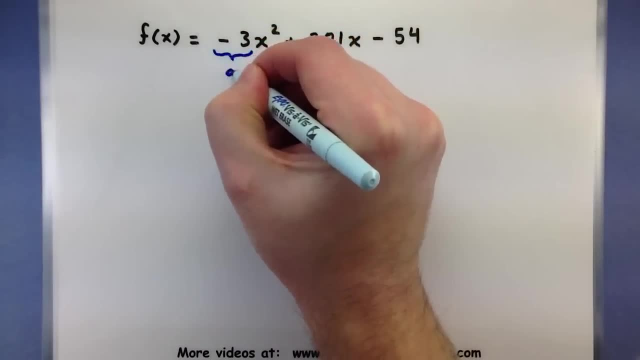 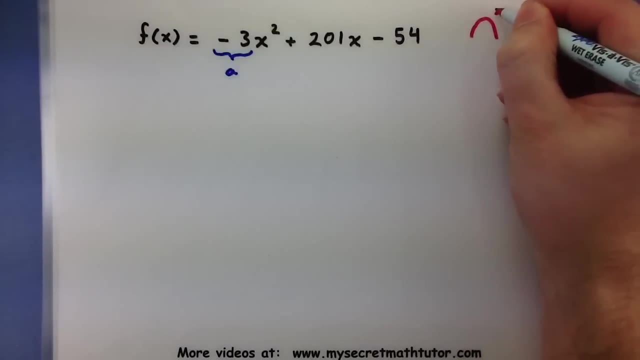 So, again, the very first thing I want to do is: let's check that a value, and in this case the a value is negative, So my parabola is facing the other way, which means I have a maximum, Not bad. 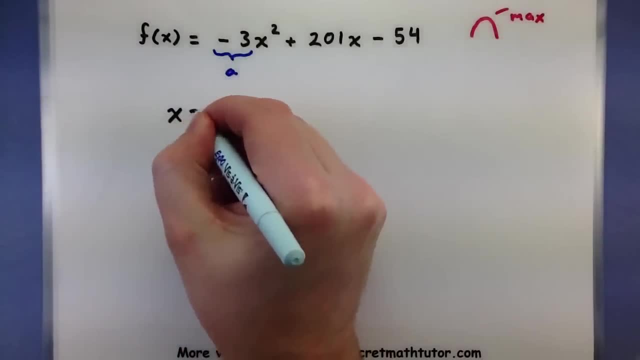 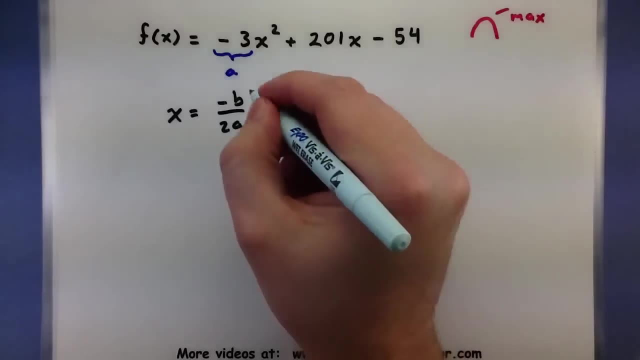 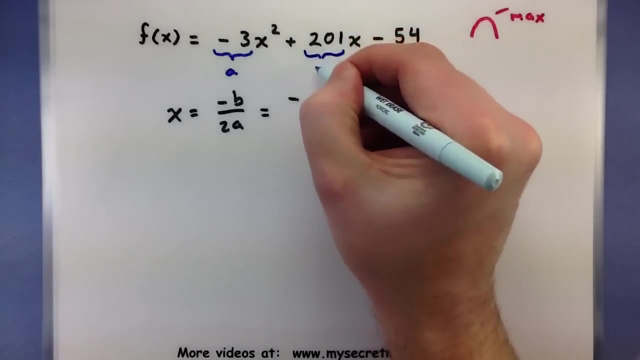 All right, now we will use our formula: x equals negative b over 2a to figure out where this happens. Okay, So negative. the value of b will be that 201, so let's grab that Negative 201 all over 2,. my value of a is the negative 3.. 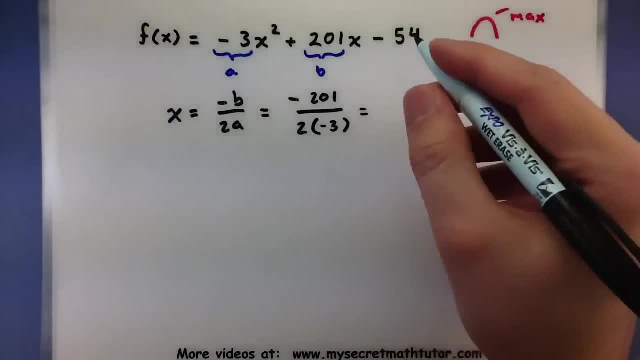 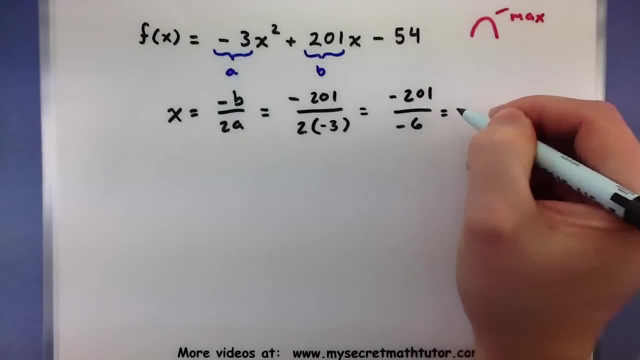 All right, looking pretty good. So it looks like I have a negative 201 all over a negative 6.. All right, I can just say 201 over 6.. Now you'll notice that this one doesn't simplify, but that's okay. 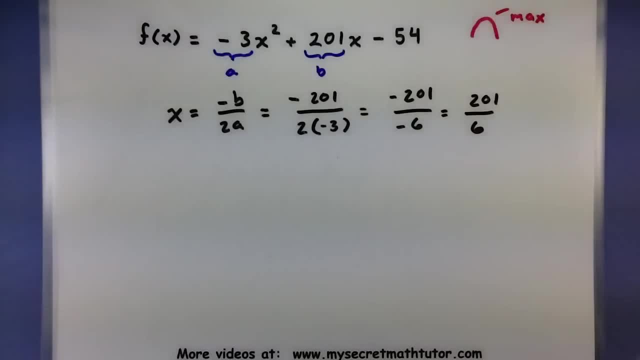 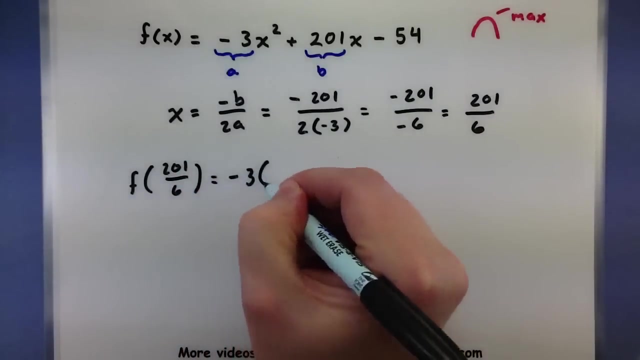 Now all we have to do is take this and plug it into our function. So, f of x, we'll plug in the 201 all over 6, and again, everywhere we see an x, we'll put in this 201 all over 6.. 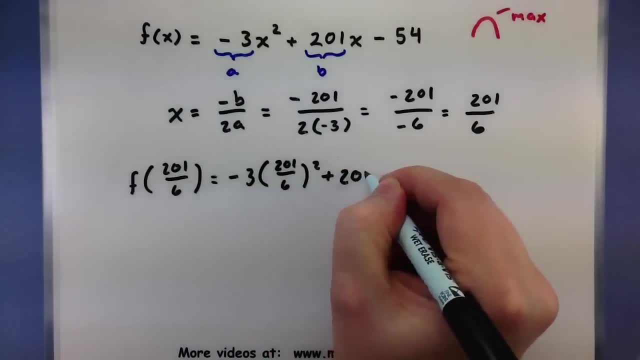 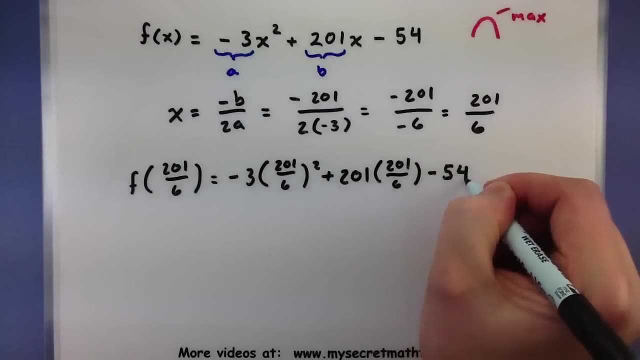 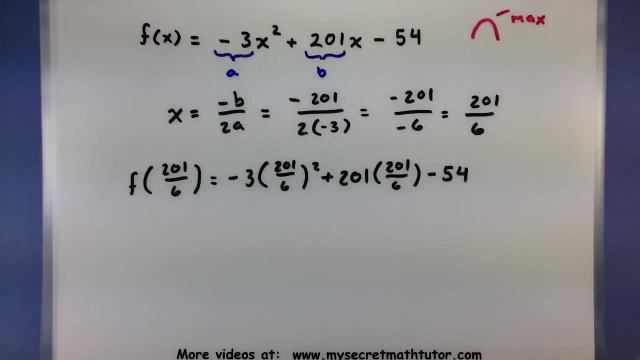 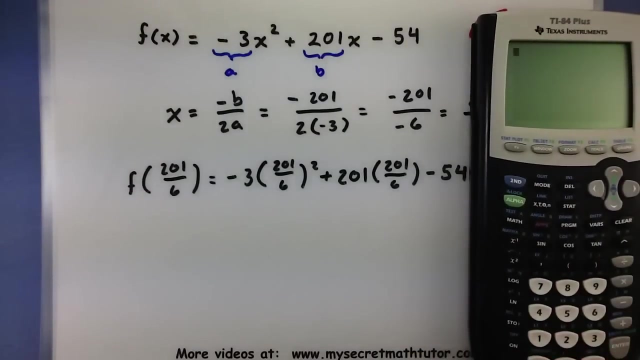 Okay, All right, So we'll plug this in Now. this one is quite a mess, so I'll definitely use my calculator to help me out as much as possible with this guy. Let's go ahead and grab it. All right, So let's plug this in. 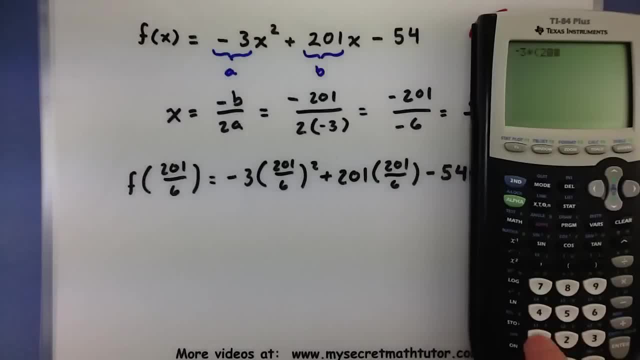 We'll start with a negative 3 times 201 divided by 6.. Okay, All right, So we'll plug it in. So we'll plug this in. This is the negative 3 times 201 divided by 6,, and then we'll plug this in. 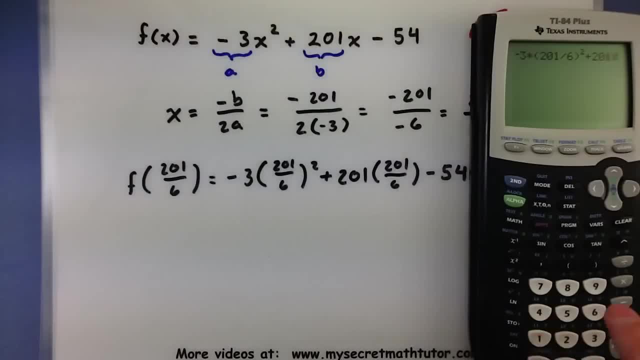 So we'll plug this in. What's this? This is the negative 3 times 201 divided by 6, squared, plus 201 times 201 divided by 6, and then minus 54.. All right, So it looks like I'm getting about 3,312.75.. 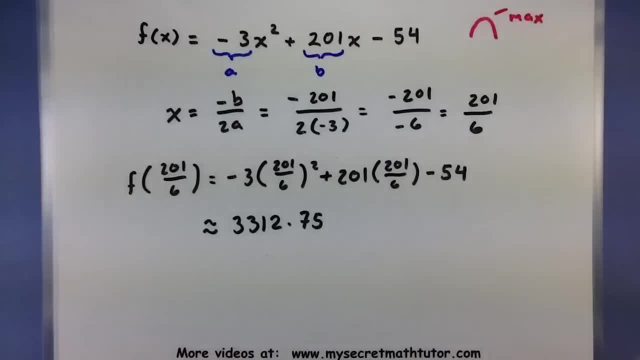 Okay, So I can say the minimum value is 3312.75.. And you can remember. if you want to know where this happens, that's the x value you found earlier. For more videos, please watch MySecretMathTutorcom.